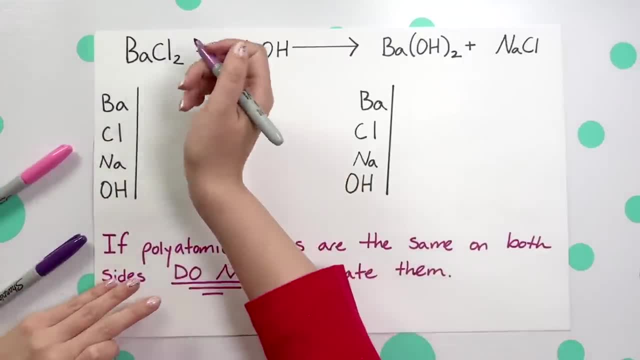 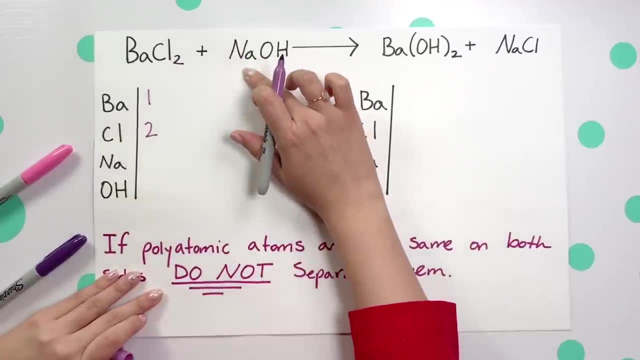 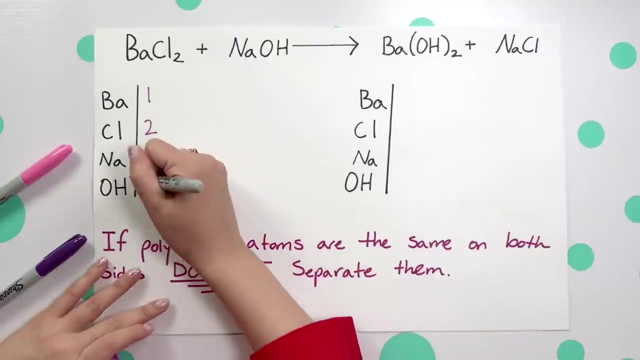 we have for our products. We have looking at barium, we only have one Chlorine. this subscript tells us we have two and A. we only have one OH has no subscript or parentheses with the subscript. so then we're just going to say that there's only one OH. Now, going to our products, we'll see that barium only. 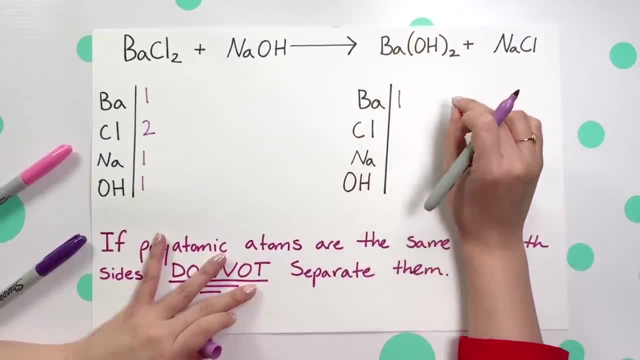 has one. Now I'm going to look at OH for right now and see that there's actually a two subscript. That two only has one, Only affects the OH group, not barium. So this is saying there are two OHs, so two OHs, and then we'll. 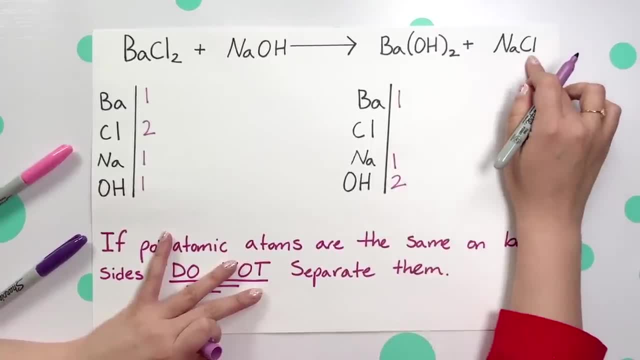 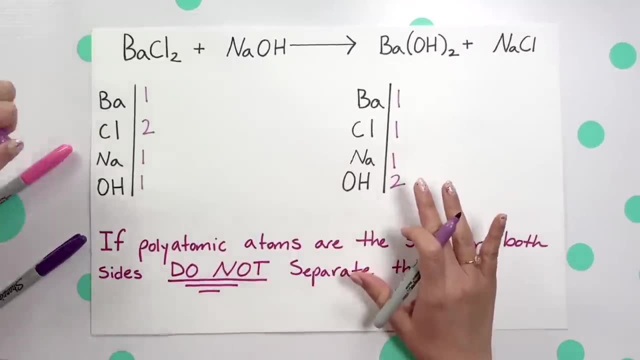 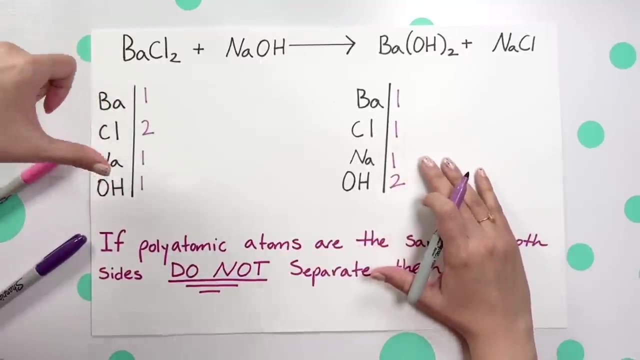 have one Na or sodium and one Cl or one chlorine. Now the next step is to figure out: okay, where are we going to start? What do we want to balance? So we have to balance out our chlorine, because there's two on this side and only one on the other, and then for OH, there's only one on our reactant side. 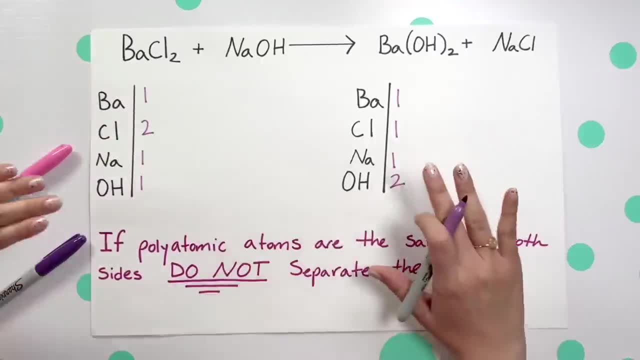 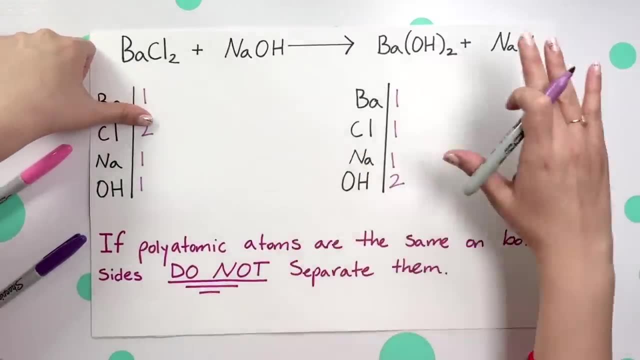 and two on. our products Always begin with everything other than hydrogen and oxygen, So I'm actually going to start with the chlorine first. So since there's a two here, I need two more on the product side. So I'm going to place a two right in front of that compound. Note that you cannot put the two in the center. 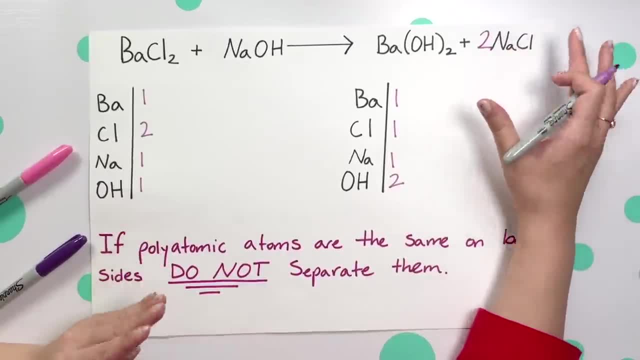 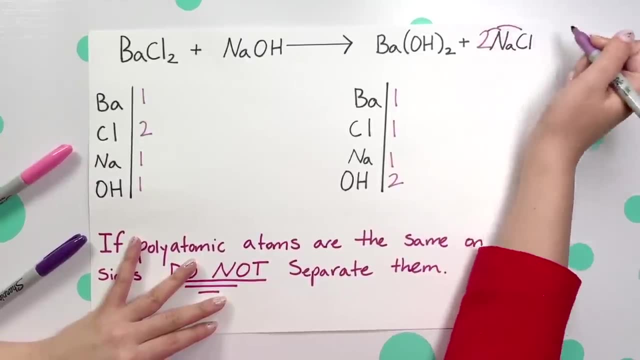 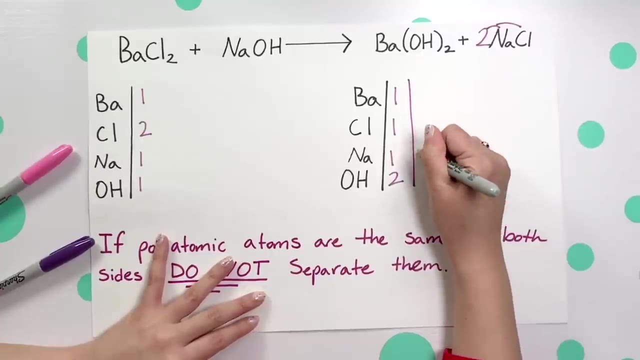 because that's then breaking apart the compound altogether and since this is a compound, this two will actually distribute and affect the Na and the chlorine. So I'm going to actually recount everything now. So if we were to recount everything, we'll see that we have two Na's and now we have two chlorine. but 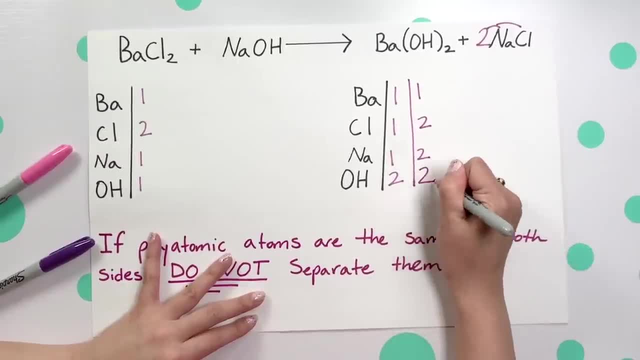 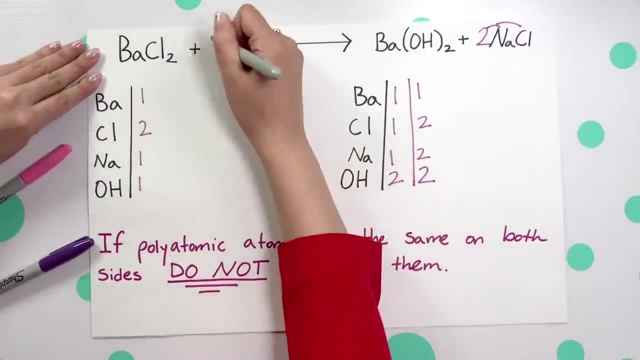 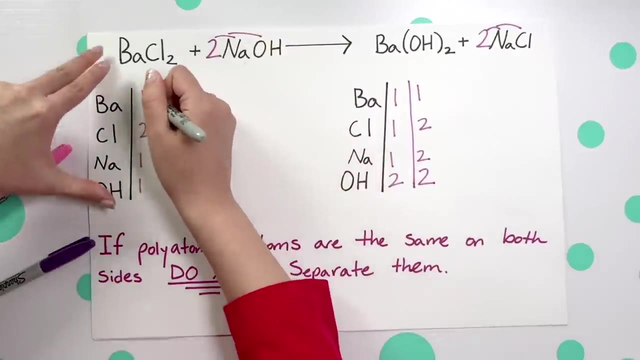 nothing changed with barium or our OH. We still have two. Now looking on the reactant side, I'm going to now continue to balance out the Na. So we need two on our reactant side. This would then distribute to both again and we'll see that this affects our Na because we now have two on that side. 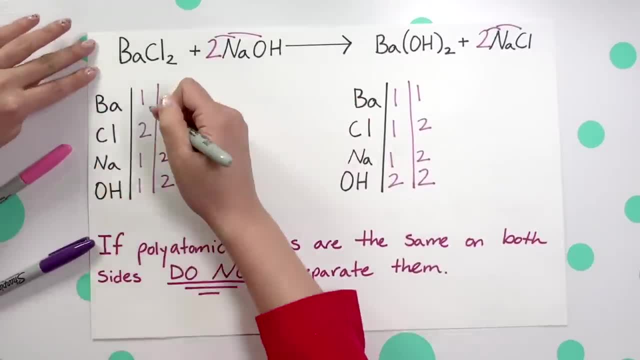 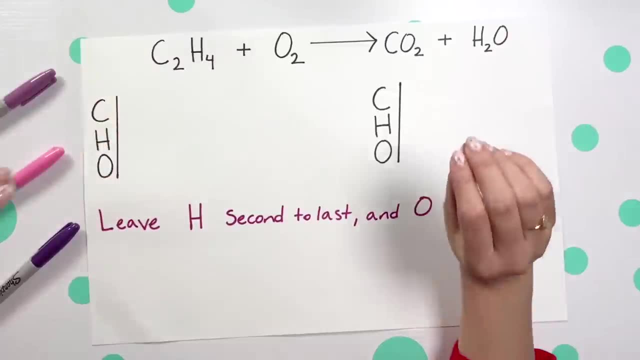 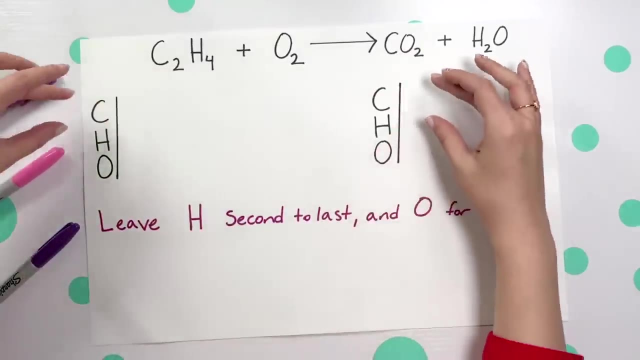 and two OHs. Everything else remain the same and we're balanced. Here we have our next unbalanced equation. Remember to start with writing all of the different elements you have for your reactant side and for your products, keeping that in the exact same order to help you balance it out Now. 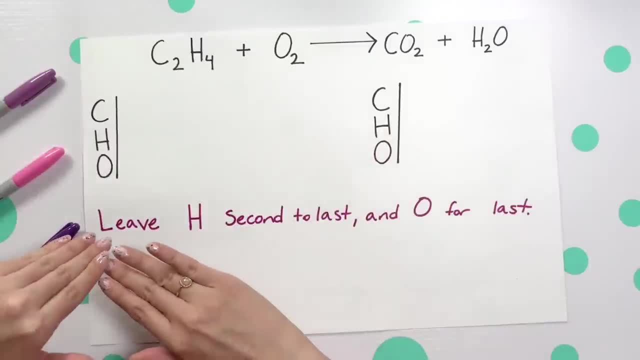 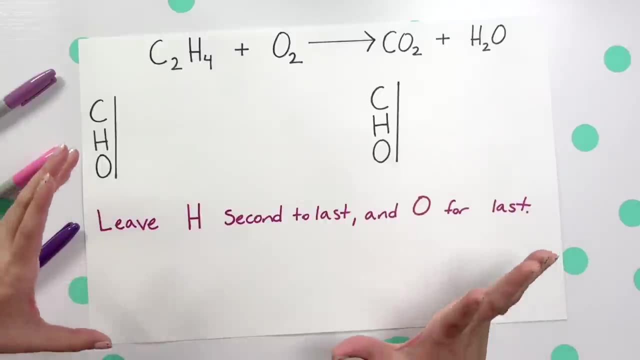 I'm always going to leave hydrogen for the second to last and oxygen for the very last. It makes it so much easier. The oxygen tends to balance out at the very end. Now, looking at this, I'm just going to count how many of each. 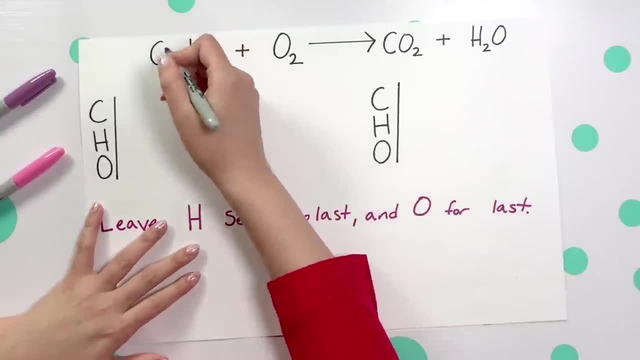 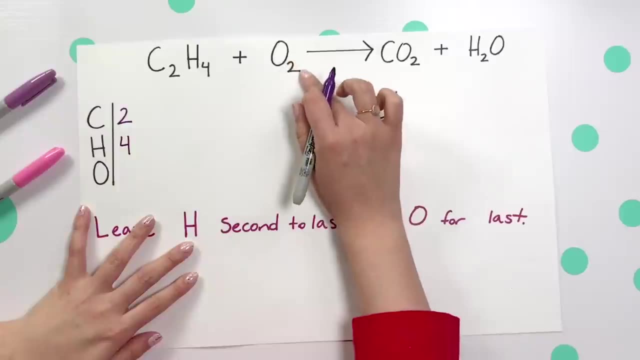 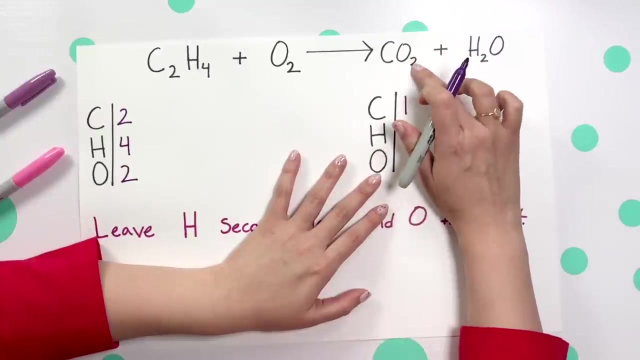 element we have. So, looking at this subscript, we have two carbon on our reactant side. Looking at the fourth subscript, we have four hydrogen and two oxygen. Now, looking on our product side, we'll see there's only one carbon. That two affects this oxygen. However, there's actually another oxygen here, so don't forget about. 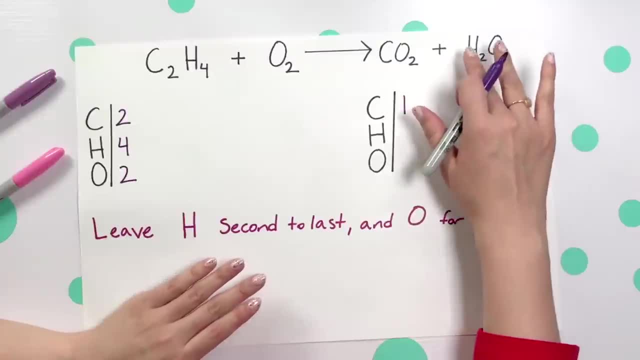 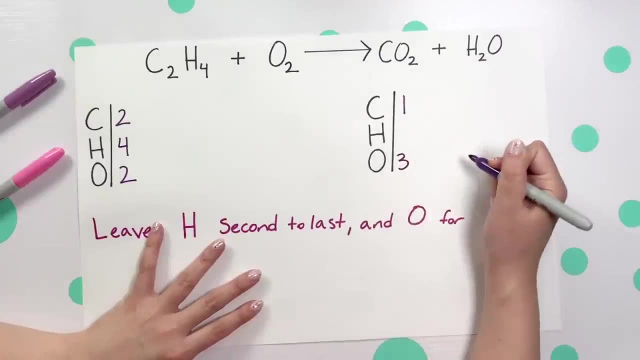 that There sometimes can be other oxygen in other compounds and I'm going to look at this and actually count it up. So there's two plus that one oxygen, making there be three oxygen on our product side. Next, we only have two hydrogen due to this subscript. 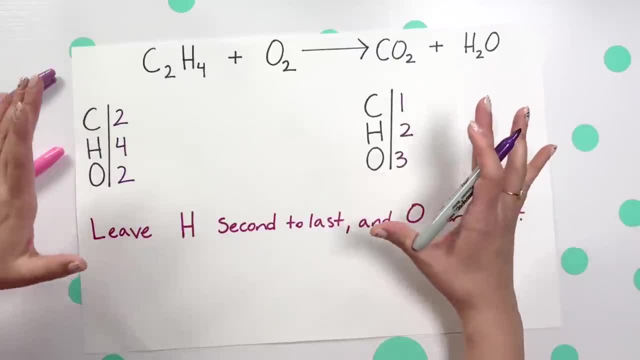 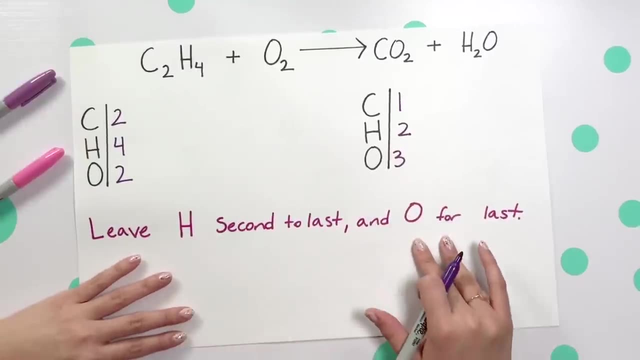 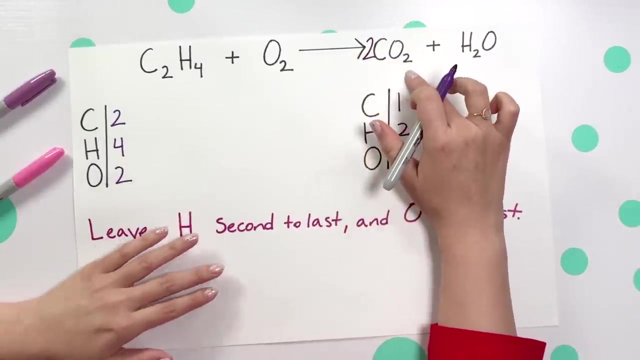 And let's look and see and relate, nothing is balanced whatsoever. We have our work ahead of us. So, looking at carbon, that's where I want to begin because, remember, hydrogen is second to last, then oxygen, So carbon- I can place a 2 right in front of that co2 compound and this affects our carbon and our oxygen because it's. 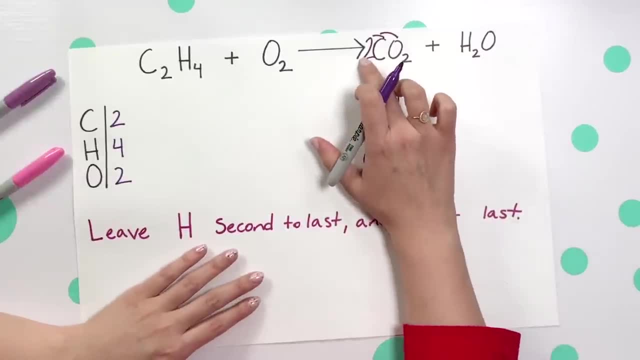 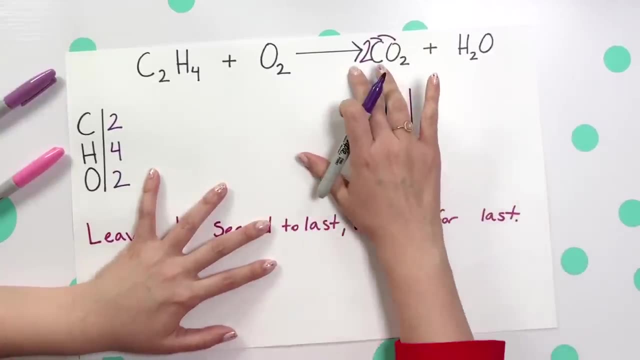 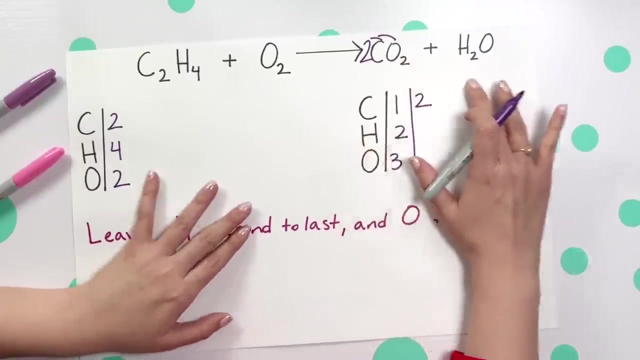 like you're distributing, and I say that because we're gonna multiply this 2 times this other 2 for our oxygen and then recount everything. so I'm going to recount and see what's affected by this 2. there's actually 2 carbon on our product side and 2 times 2, so 4, 4 plus this other 1 oxygen. 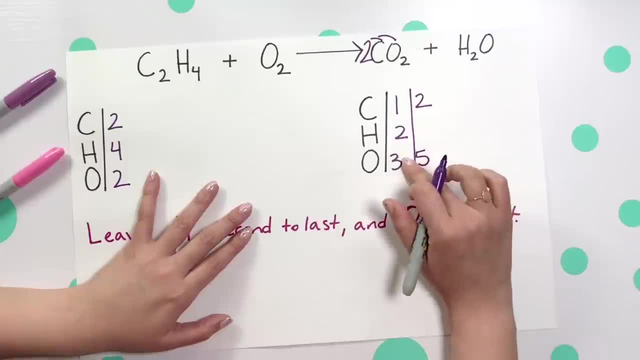 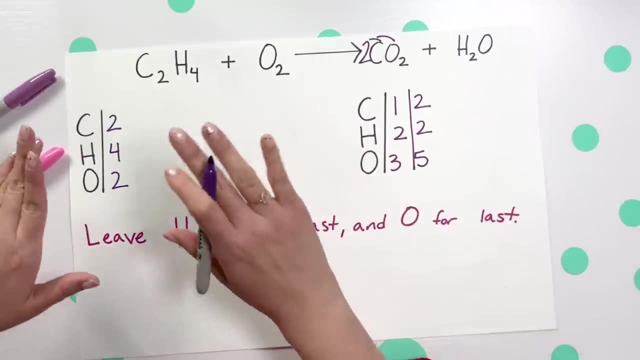 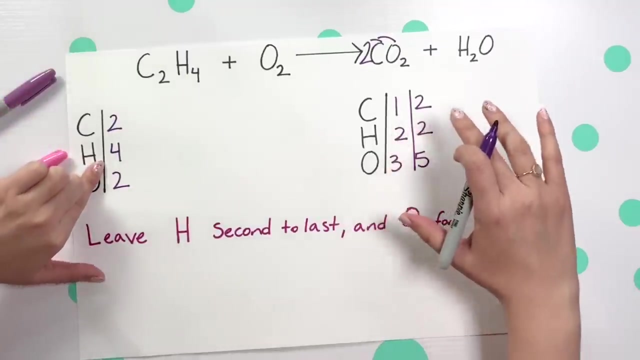 making it 5. so we now have 5 oxygen on our product side and nothing happened with hydrogen, so that stayed the exact same. now let's go back to our reaction side and then we'll balance out our hydrogen. so we'll see there's only 4 on this side and we have only 2 on our product side. so I